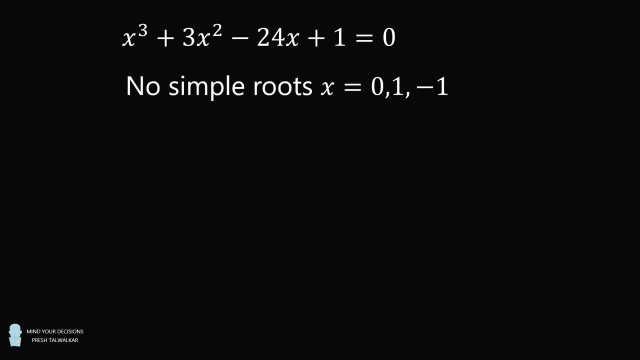 cubic equation. There are no simple roots like x is equal to 0, x is equal to 1, or x is equal to negative 1.. There's also no obvious way to factor the cubic equation, So we want to think about other. 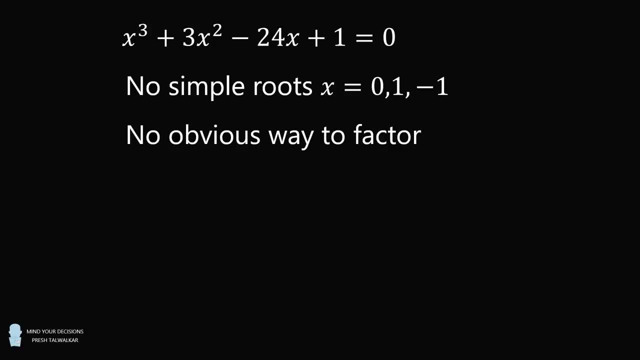 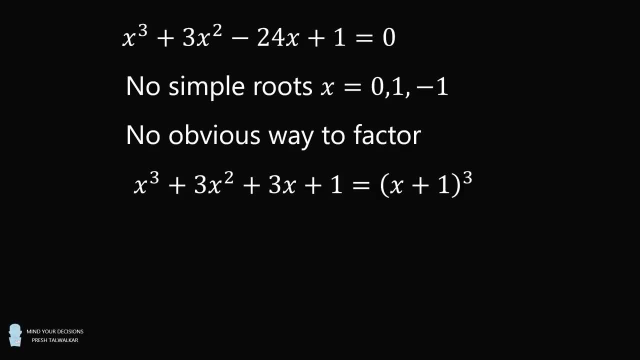 plus 1, which is equal to the cube of the sum x plus 1.. So let's transform the original equation by adding 27x to both sides. The left-hand side then becomes x cubed plus 3x, squared plus 3x plus. 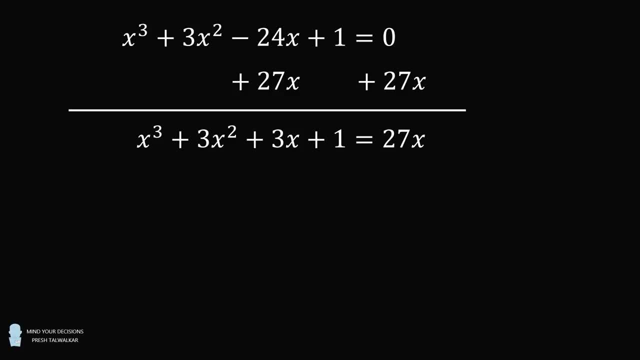 1, and the right-hand side is 27x. The left-hand side factors. We can then take the cube root of both sides and the cube root of 27 is equal to 3.. So we have: x plus 1 is equal to 3 times the cube root of x. 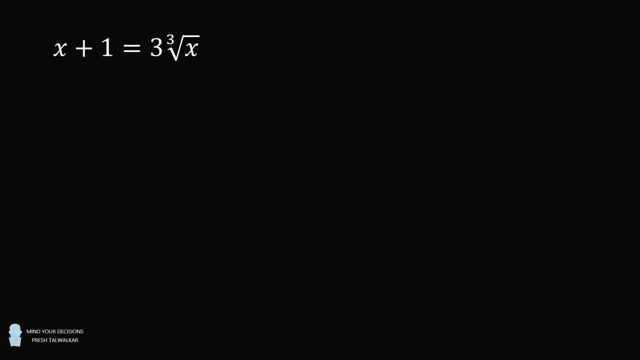 Now, alpha, beta and gamma are roots of the original equation, which means they satisfy this equation as well. Alpha plus 1 is equal to 3 times the cube root of alpha. Beta plus 1 is equal to 3 times the cube root of beta. and gamma plus 1 is equal to 3 times the cube root of alpha. 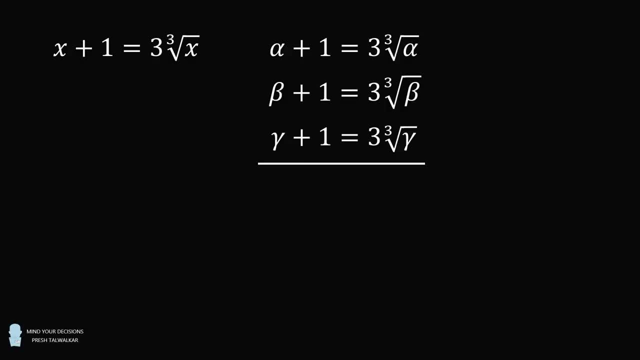 gamma. Let's now sum these three equations together. We get alpha plus beta plus gamma. plus three is equal to three times the cube root of alpha plus three times the cube root of beta plus three times the cube root of gamma. Let's factor the right hand side and then divide both sides by: 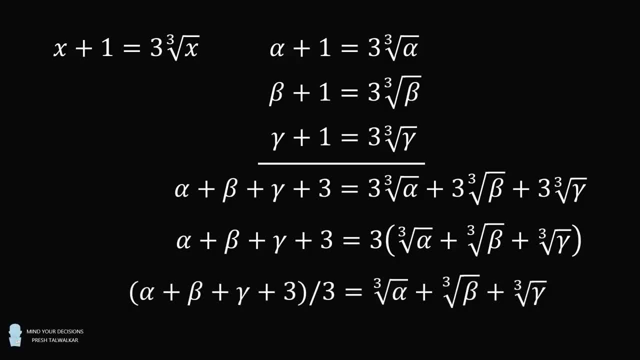 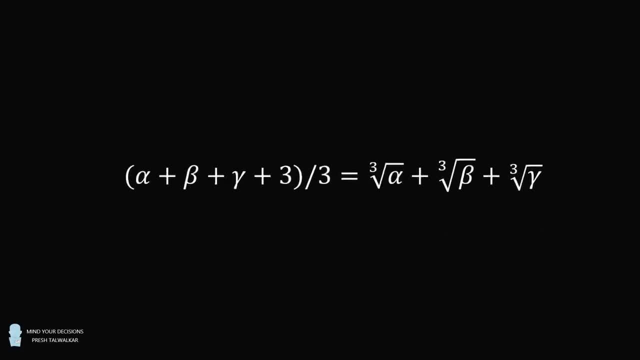 three. So we're making good progress. We now just need to figure out the sum of alpha, beta and gamma, But we can do that From the original equation. we know that negative the coefficient on the second highest term divided by the coefficient on the highest term will be equal. 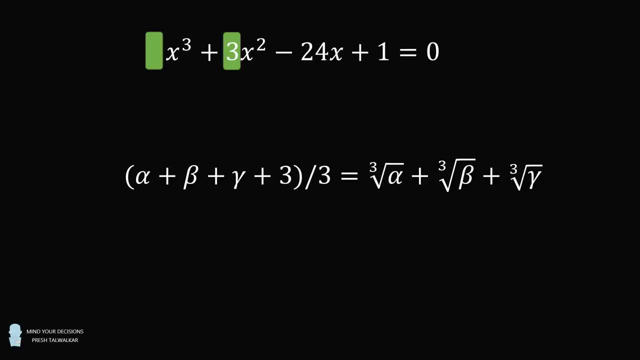 to the sum of the roots. The roots are alpha, beta and gamma. So we have: alpha plus beta plus gamma is equal to the opposite of three over one, which is equal to negative three. So alpha plus beta plus gamma is equal to negative three. We can substitute that in and then we have negative.